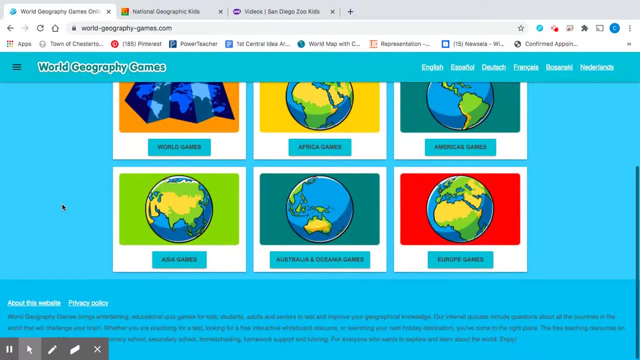 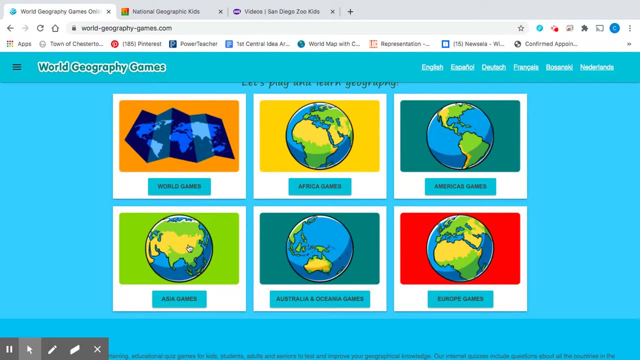 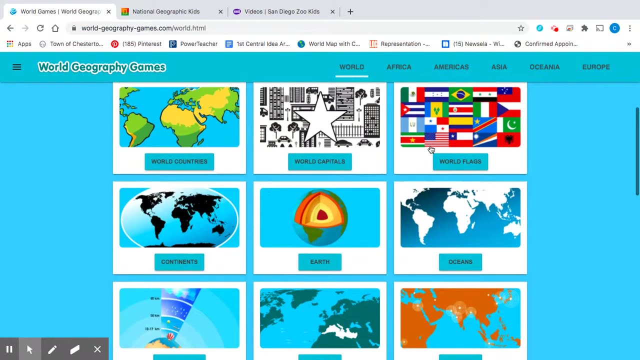 your grade about this website. So we have games for all over the world. You have World Games, Africa Games, Americas and North and South America, Europe, Australia, Asia. Let's go to World Games. Learn about world countries, world capitals, the flags of the world, oceans, that. 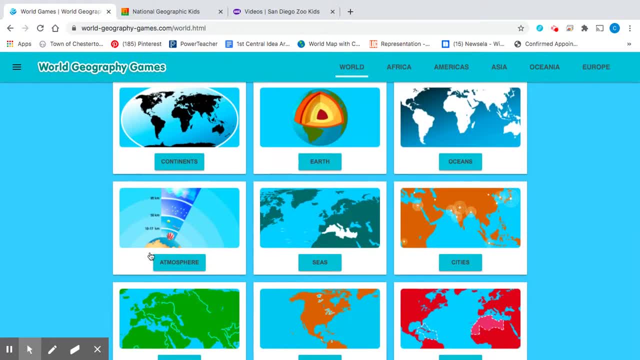 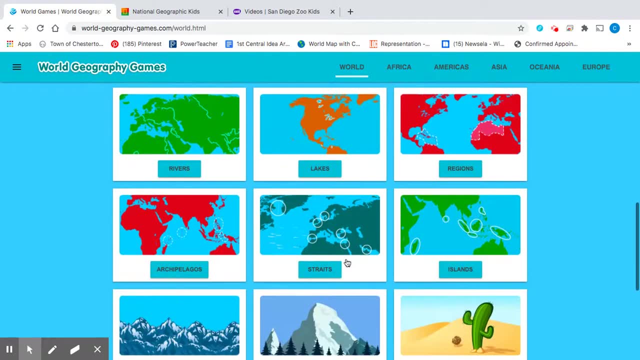 make up the world: the earth itself, continents, the atmosphere. So a little bit of science in there. The seas, cities, regions of the world, the lakes, straits. So straits are just like a different kind of body of water. You can learn about islands, the deserts of the world. 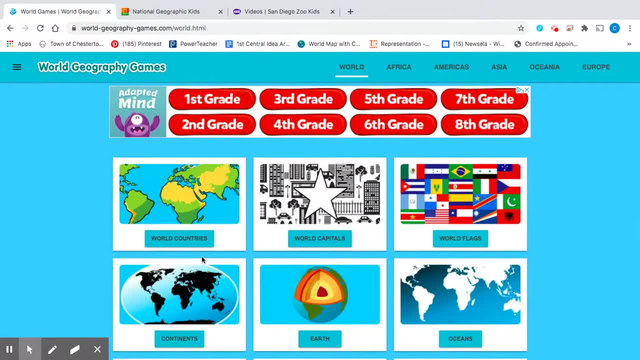 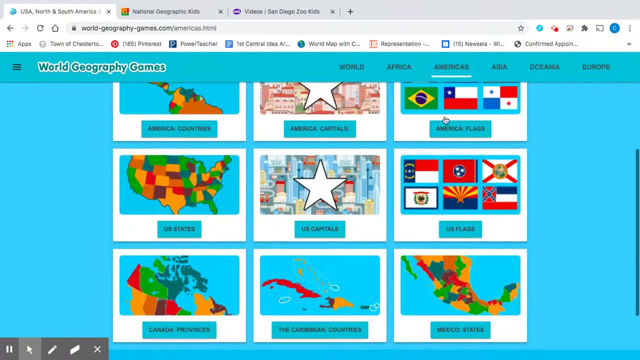 the mountains of the world, volcanoes, all this different, really cool stuff. Let's say we want to learn about the Americas, So we go here. we can learn about the flags in America- And this just breaks it down even more- from World Games. Learn about the capitals in. 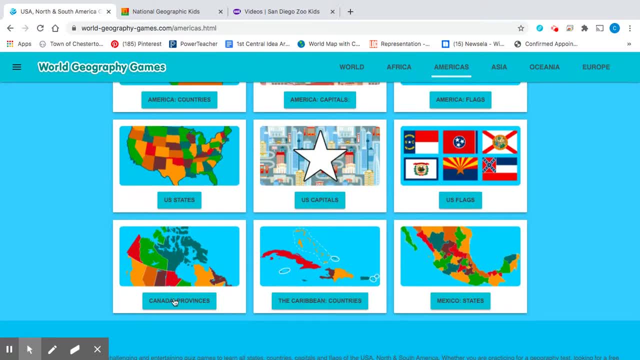 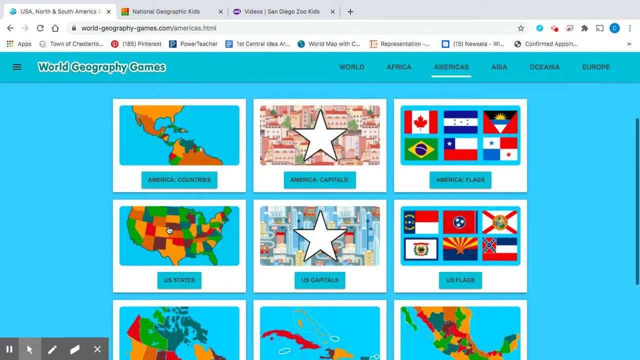 the United States, the countries of the Caribbean, the areas that make up Canada, the provinces, as they're named, the countries that are in America, the states that make up the United States. Like I said, let's see. let's. maybe we want to go to eighth grade. Let's see what we can learn. 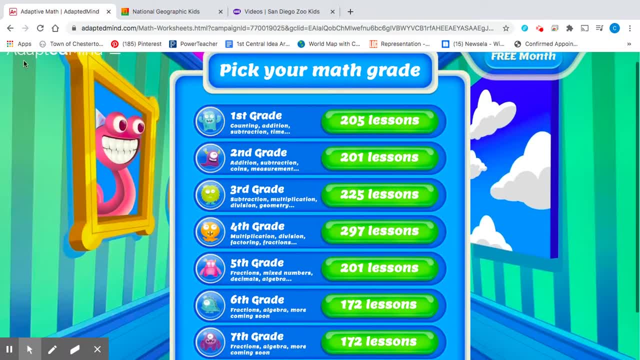 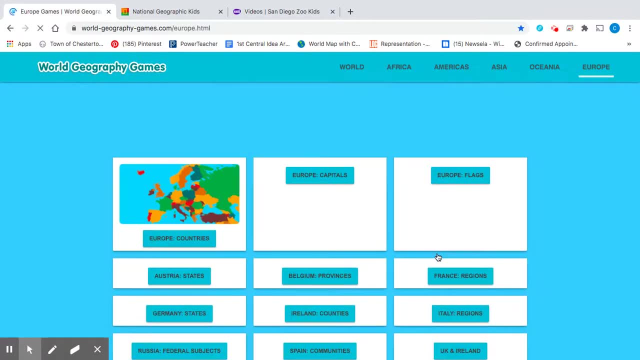 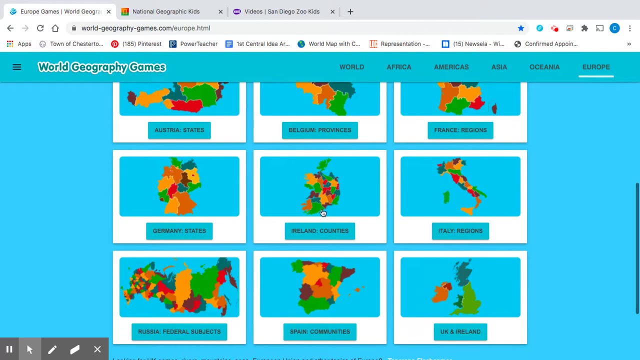 about eighth grade. Oh, it's actually a different website. Nevermind, If we go here, let's go back to. we can go to Europe Games Again. it breaks it down even more. You can learn about regions of Italy, the regions. 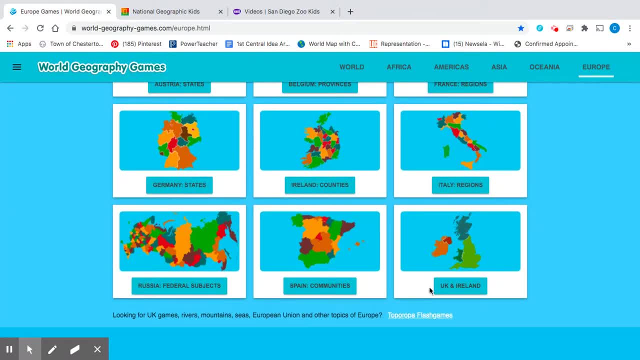 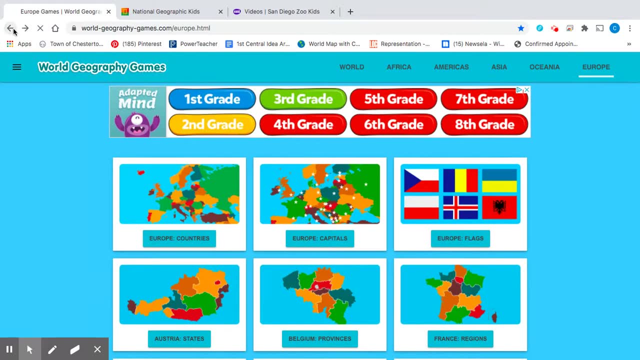 of Ireland, Spain, So these are all different countries in Europe. You can learn about the United Kingdom in Ireland, Russia, the areas of Russia, the countries that make up Europe. So you guys can use this website just learn about more about the geography and how you know. 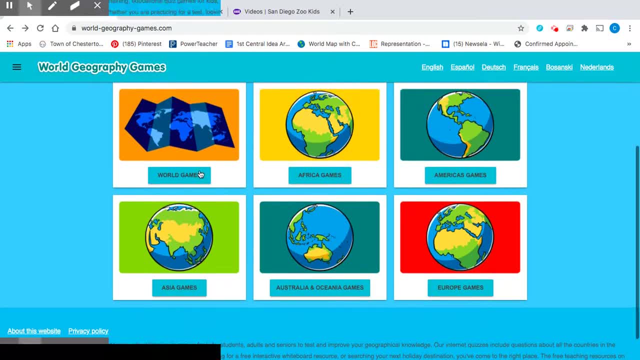 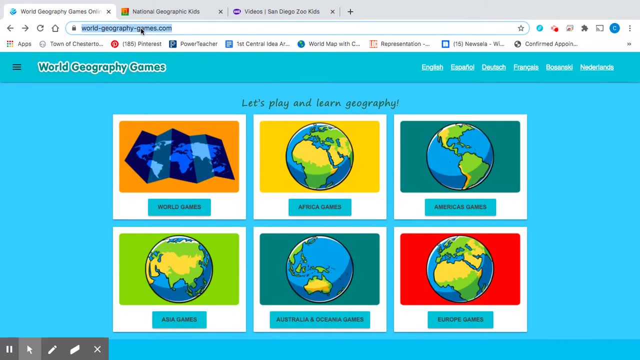 different parts of the world are made up, what they look like, what is in them, what the people were like there. So World Geography Games guys is another website you guys can use to further your understanding of geography around the world. If you have any questions, please let me know.